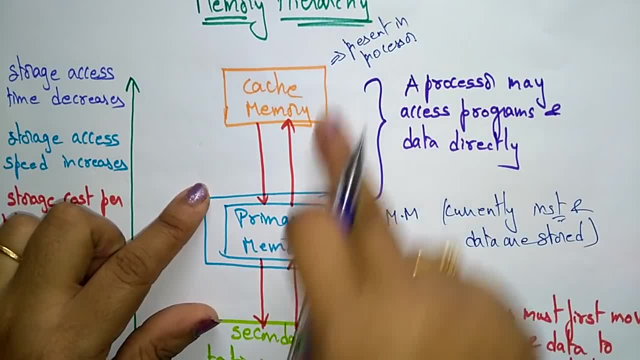 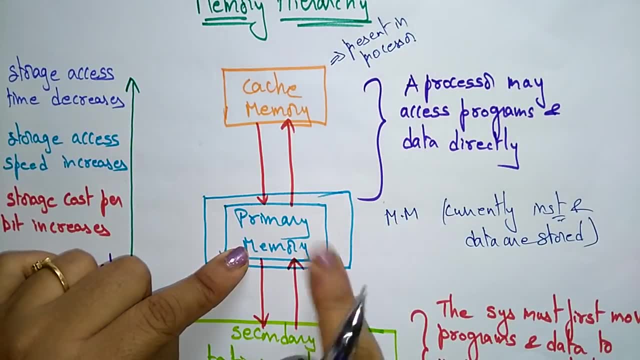 totalement file to fschoolse. A processor can access programs and data directly in the main and cache memory. A processor can access here in the main and cache memory Am Wireless, Am Wireless. So here the present data that has to be accessed will be stored in cache and the main memory. currently instruction and data are stored in primary memory. 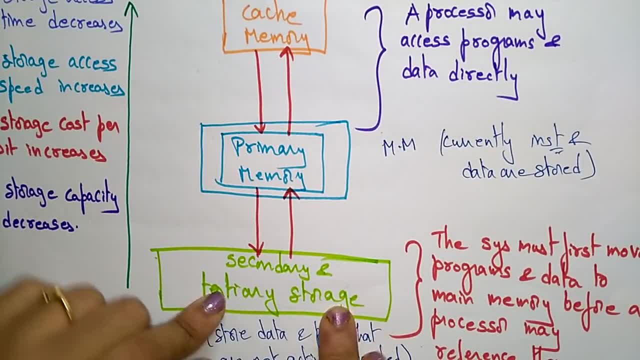 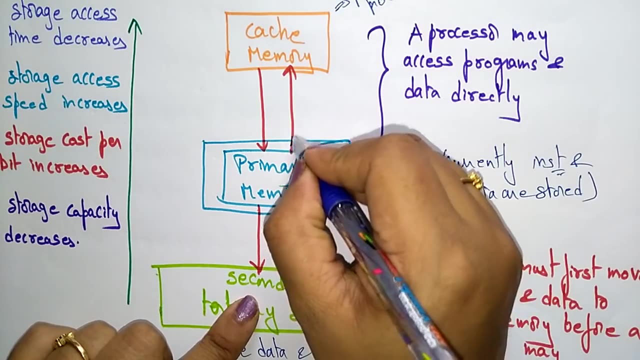 And the secondary storage. the system must first move programs and data to main memory before a processor may refer them. Before a processor may refer them, that complete program will be transferred to the primary memory. The secondary will transfer to the primary memory and only the current instruction that has to be executed that will be stored in cache memory. 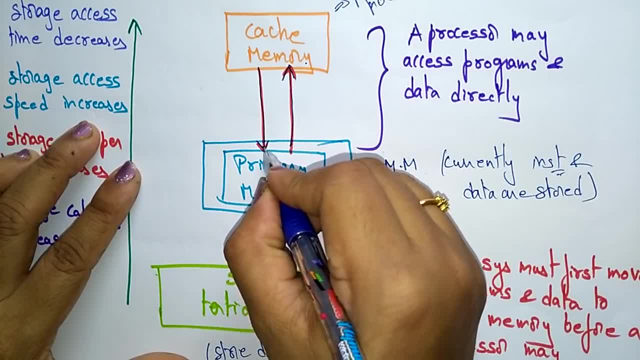 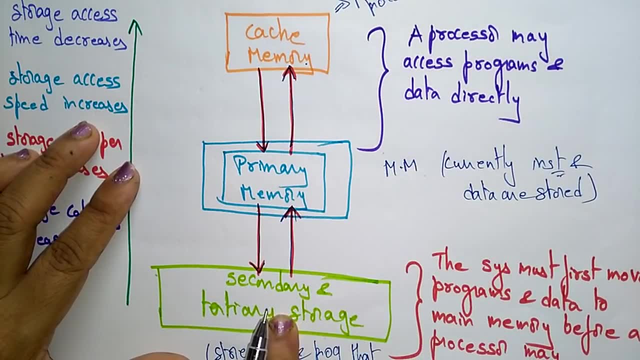 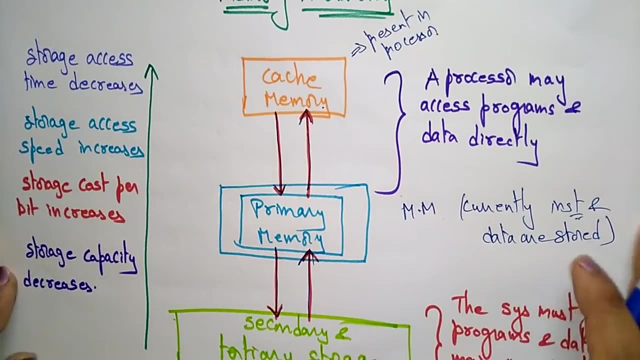 And again, the result of the current instruction will be stored in primary memory and the primary memory will send that complete the executed data to the secondary storage. So this is how the operations will be done, So in the memory hierarchy, while going from down to up. 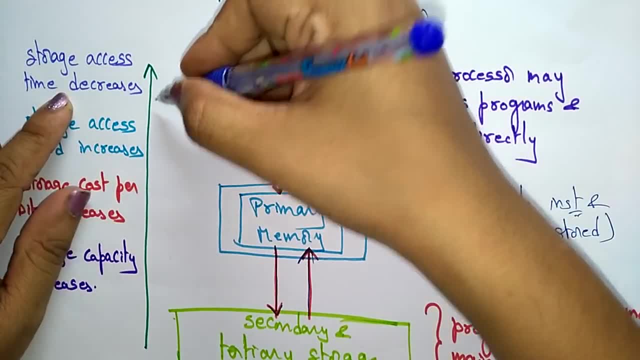 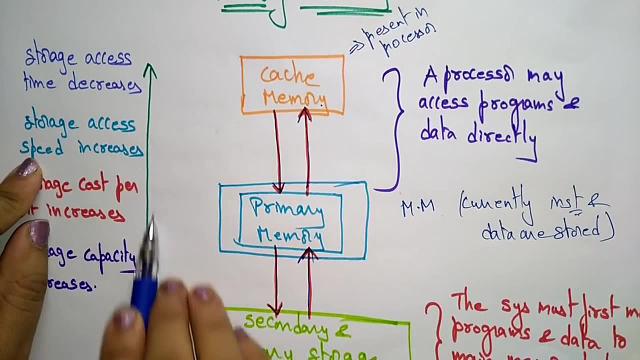 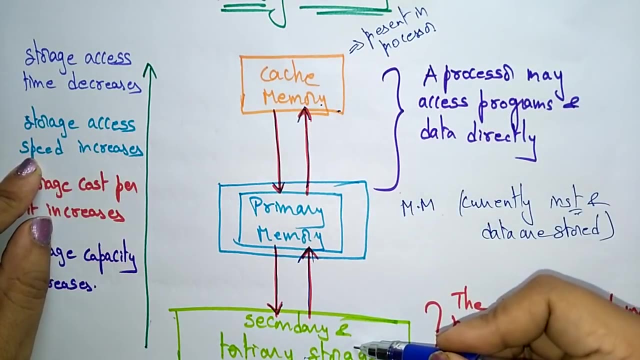 Means from bottom to up. The storage access time increases. The access time is increasing Storage access time. Storage access speed increasing. The speed is increasing When compared to the secondary. the cache is having the more the speed of the cache is more when compared to the secondary. 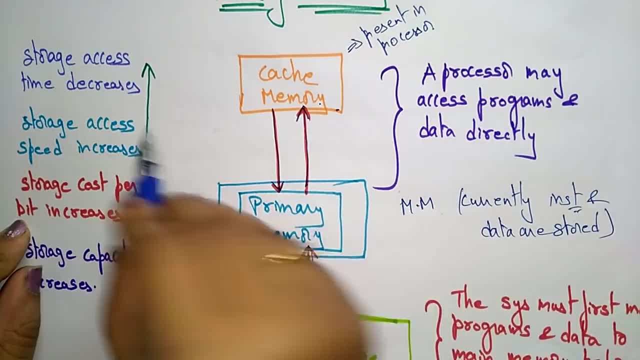 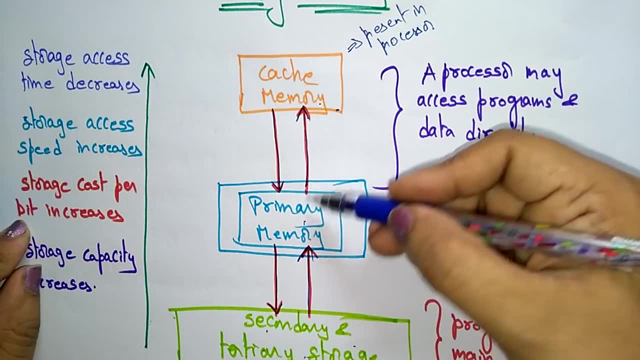 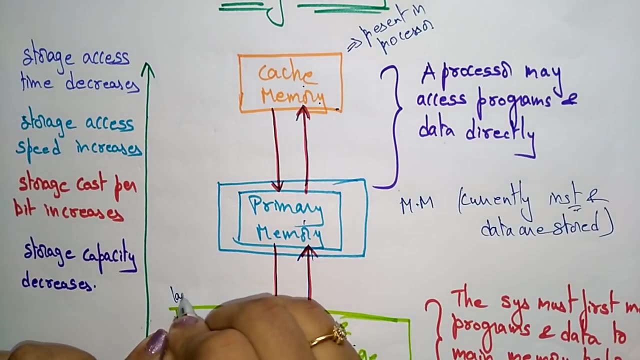 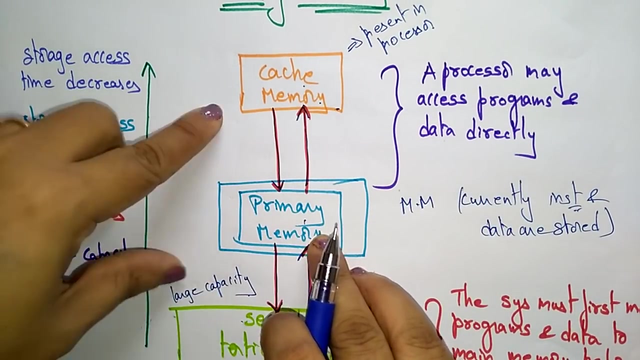 And storage cost per bit is also increasing, So here the cost is also increasing. Secondary, when compared to primary, is most cost effective And The cache is more expensive And storage capacity decreases Here. this is having the large capacity. Okay, And this is the small, and compared to primary, the cache is a very small storage device. 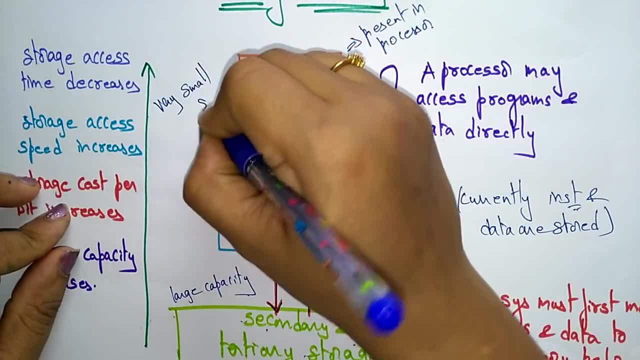 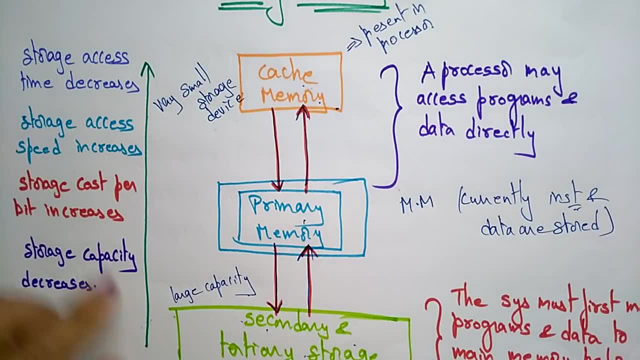 So this is very small storage device, Storage device. So while going from bottom to up, the storage capacity is decreasing. So these are the features of this memory hierarchy. So the main thing You have to be remember that Suppose whatever you have taken, 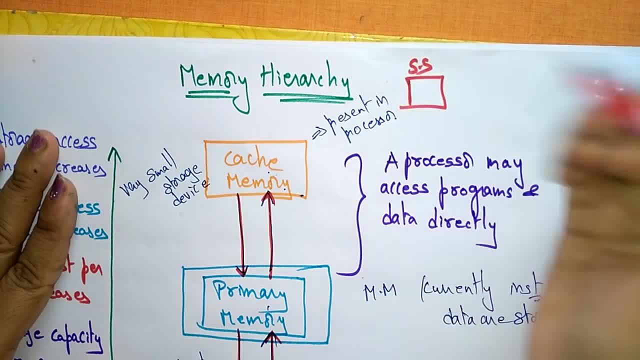 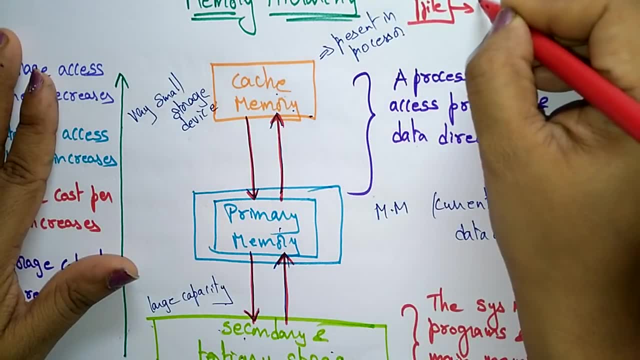 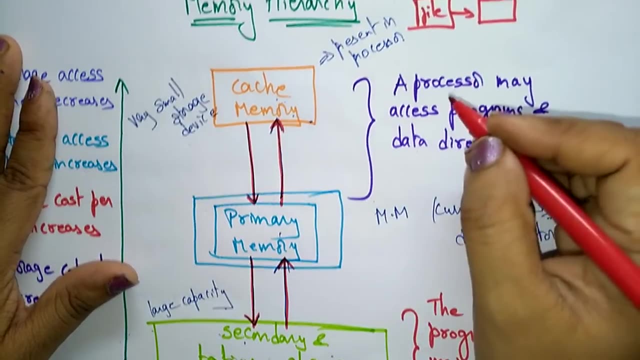 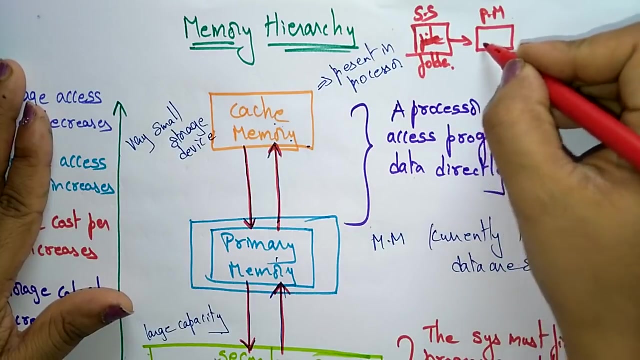 This is the secondary Storage. A secondary storage contains complete file, So that file will be transferred to Only the Primary memory. Okay, So suppose this is the folder. A folder is mode, So in the primary memory the folder will be mode to the.